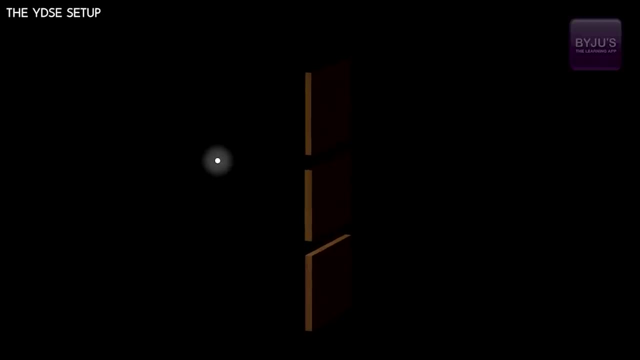 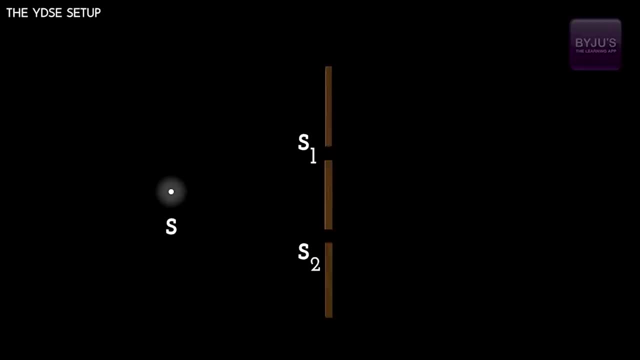 just two points: S1 and S2.. And, of course, on the other side there's a screen. Now, one thing to note is that the point source S is placed in such a way that it is equidistant from S1 and S2.. Okay, Now what would happen? Now we know that the point source S- because 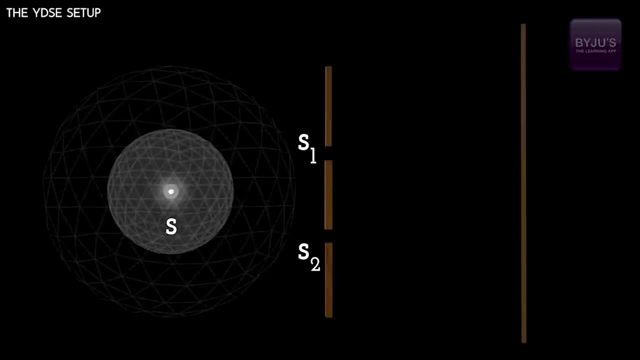 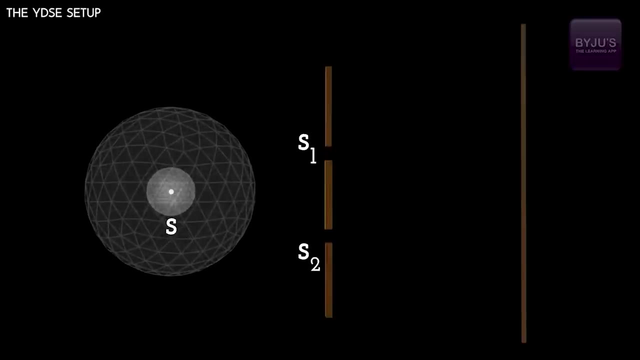 it's a source of light, it'll produce spherical wave fronts. Now, when these wave fronts, when they hit the slits S1 and S2, what will happen? So we know that from half a second, S1 and S2 will hit the slits And S2 will hit the 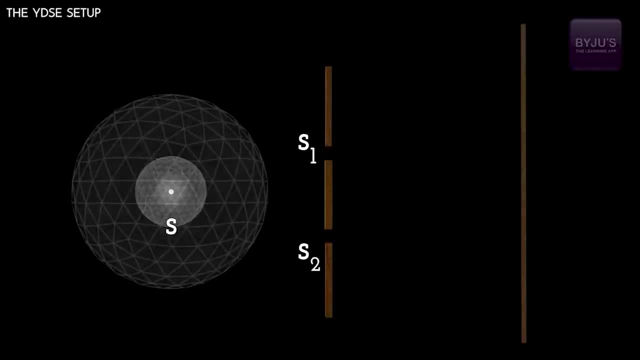 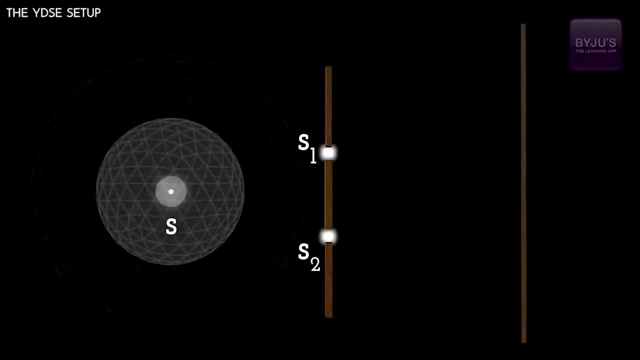 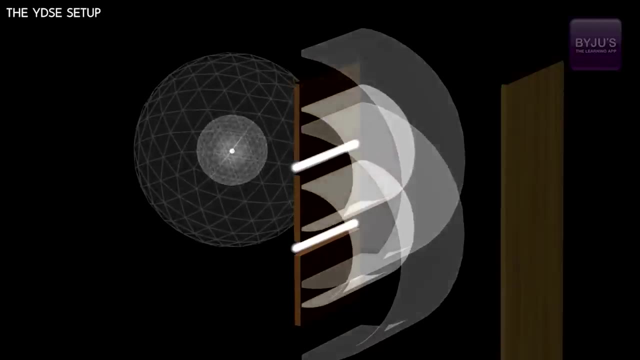 as a source itself. So, therefore, these two slits will produce cylindrical wave fronts. In fact, if you look at the front view, these wave fronts will look like this Right, And from the side view, if you consider a plane of cross-section, they'll basically look: 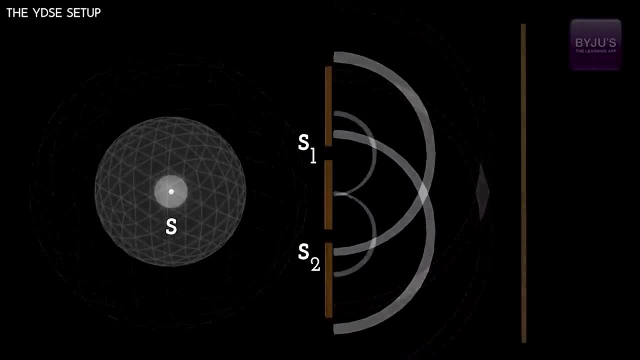 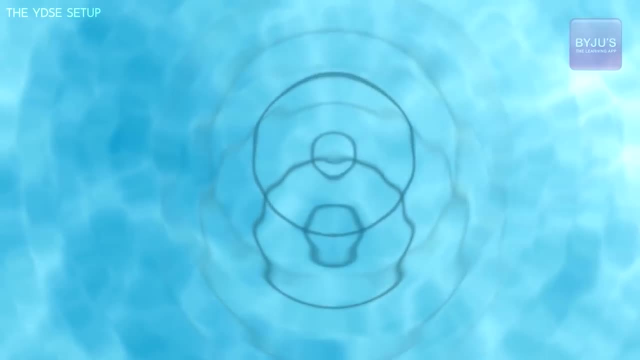 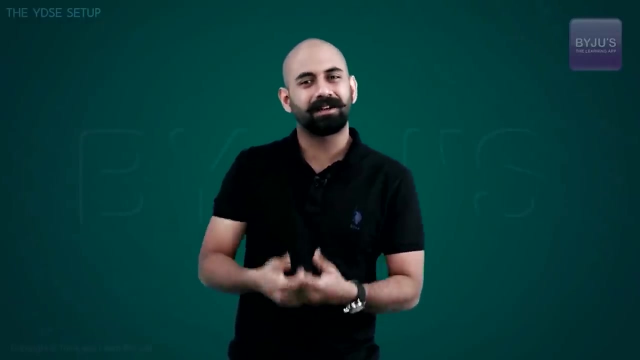 like this. You can see that these wave fronts will look like circles that are expanding Right, Very similar, in fact, to ripples on a calm surface of water. Now, the obvious question is what happens when these wave fronts intersect, when they touch? 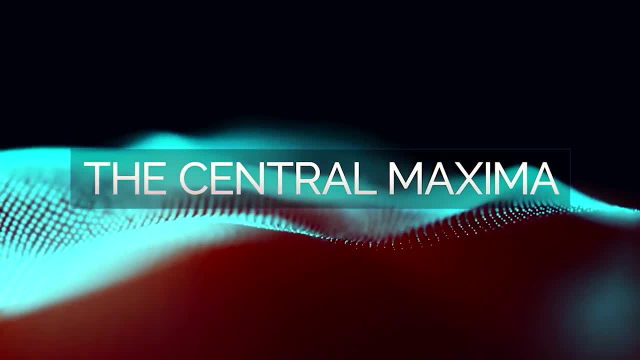 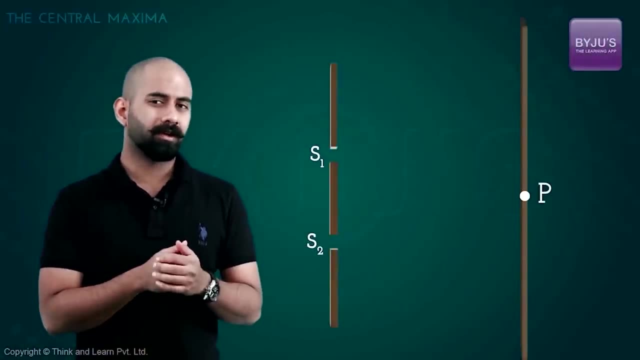 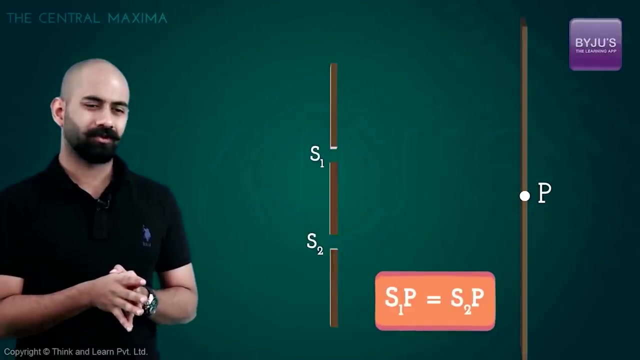 They will interfere. So now let's consider a point on the screen P which is equidistant from S1 and S2. What would happen over there exactly? So obviously, because S1 and S2 are the sources. they will produce waves, but there will be. 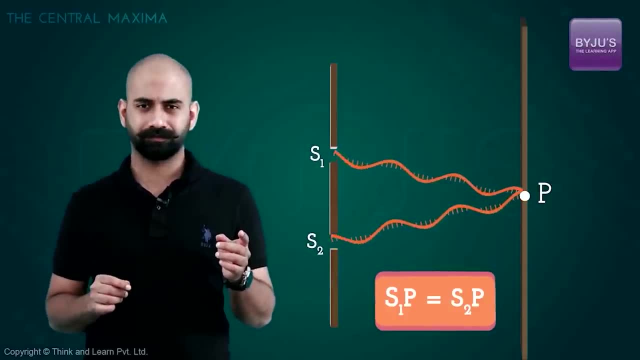 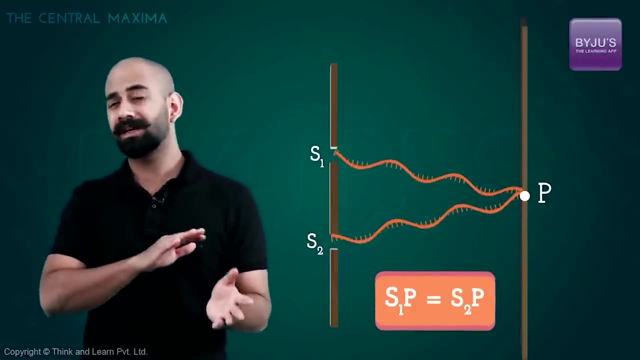 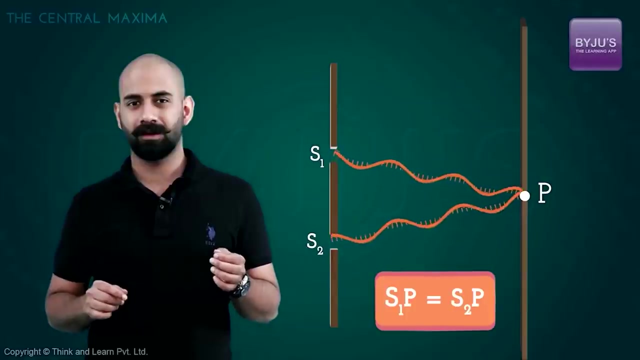 only two waves that reach P, one from S1 and one from S2. So S1 and S2, in fact, will produce infinite waves in all directions. but we don't really have to worry about all that. We only have to worry about the waves that are reaching P from S1 and S2.. 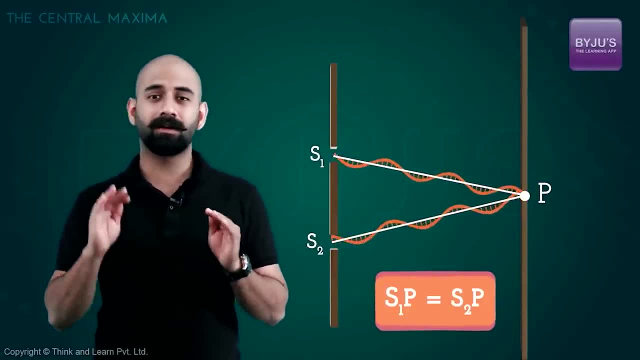 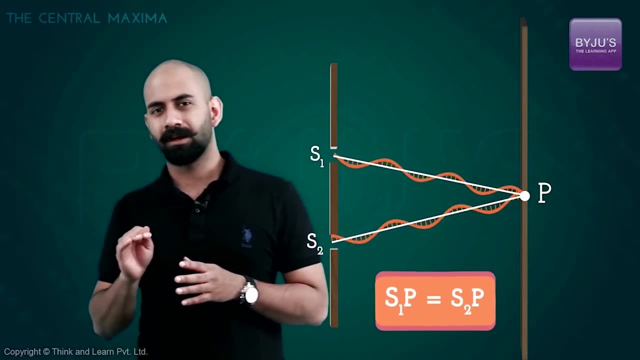 So if I draw a line S1P and S2P, I am only worried about those two waves that are coming from S1 and S2.. Let's also analyse these waves a little. First of all, these waves are electromagnetic waves. 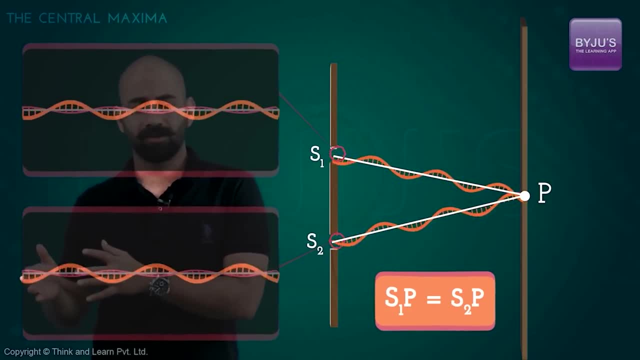 They are not mechanical waves like the ones we considered in the previous case, So they are basically waves of varying electric and magnetic field. So, of course, let's not worry about the magnetic field right now, So let's only talk about the electric field. 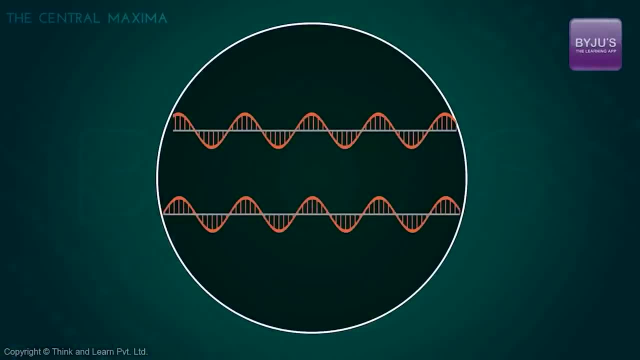 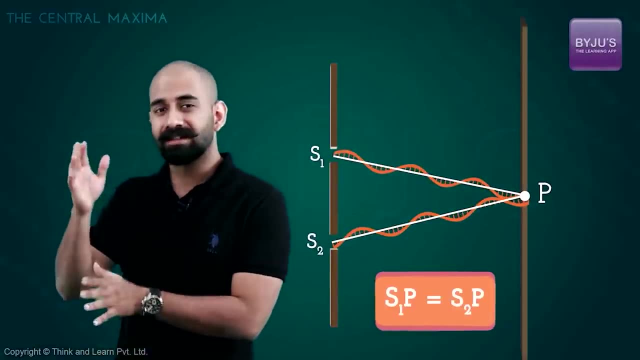 They are waves of varying electric field. Let's say that the amplitude of both these waves, Let's say that the amplitude of both these waves Is the same and let's call it E0.. Also, when they start from S1 and S2, they will be in phase because they are equidistant from. 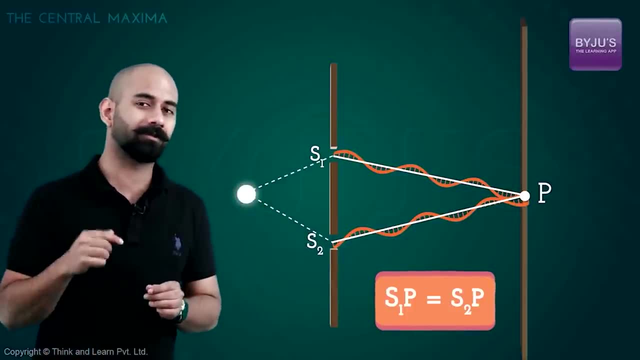 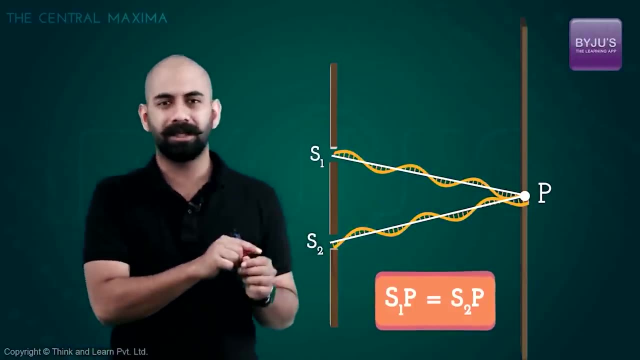 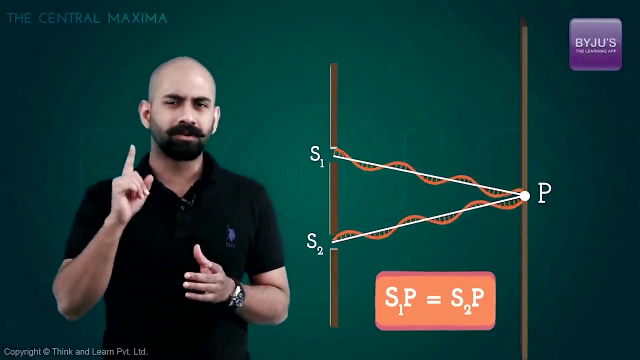 the source. So from the waves that start from S1 and S2, they will start in phase. Now, what will happen when these waves reach the point P? It will obviously interfere because there are two waves intersecting at the same point. So this is slightly different, again, from the previous case. 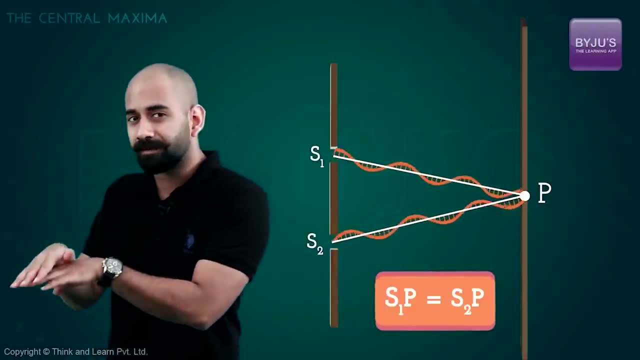 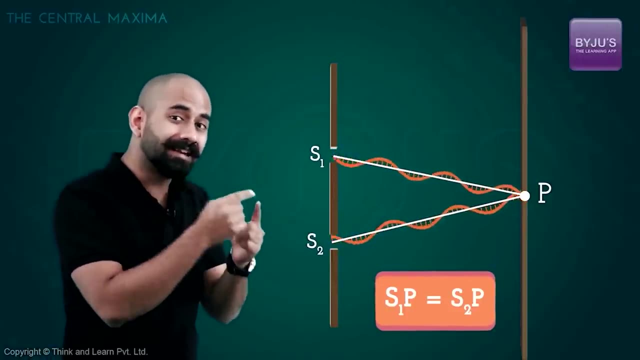 In the previous case We considered two waves that are traveling in the same string, But this is analogous to two waves that are traveling in two different strings that are intersecting at one single point, So the interference will still occur at that same point. 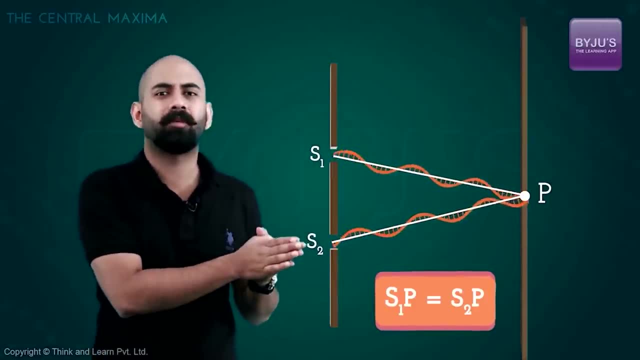 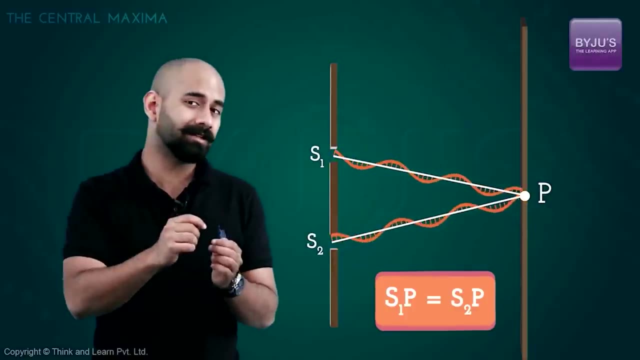 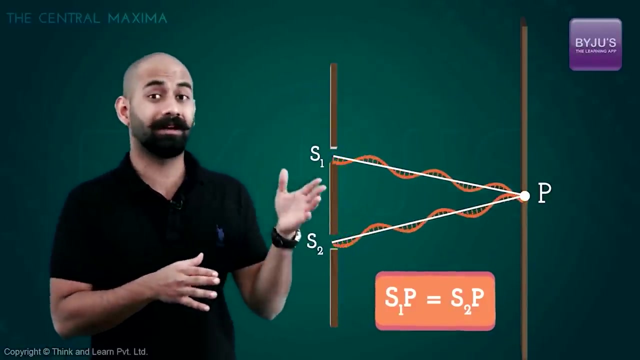 So if I had a device that measured the electric field at that point, what would it measure? It would basically measure the sum of the individual electric fields contributed by both these waves. Okay, Fine, And what would be the amplitude of the electric field at that point? 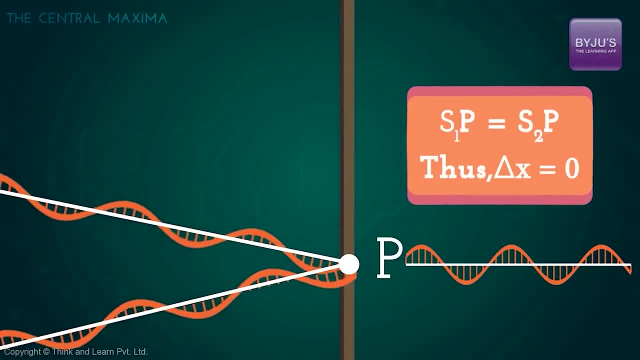 Now that depends on the path difference. What is the path difference between these two waves? It is zero, because you can see that S1P should be equal to S2P. So if the path difference is zero, then they will basically reach in phase at that point. 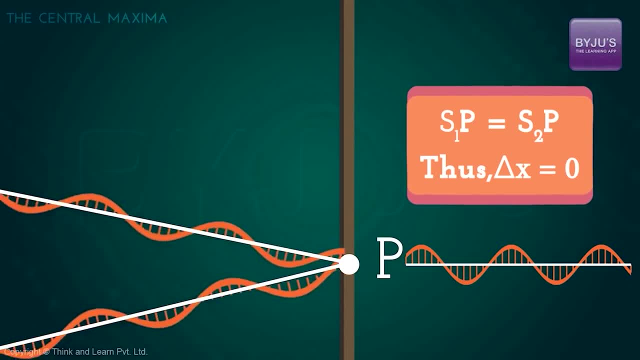 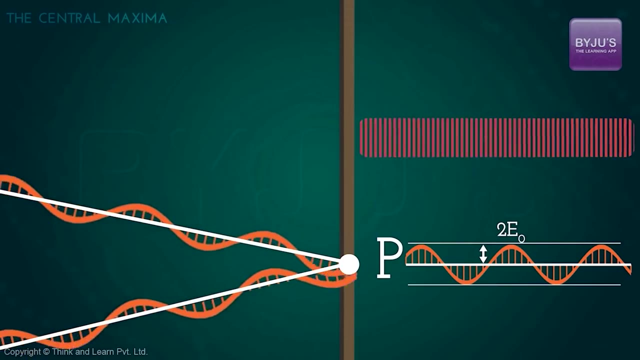 P, So at every single point in time, the resultant field will be twice the field contributed by each of these waves, Because they are in phase. So therefore the amplitude will be 2E0.. And what kind of interference is this? 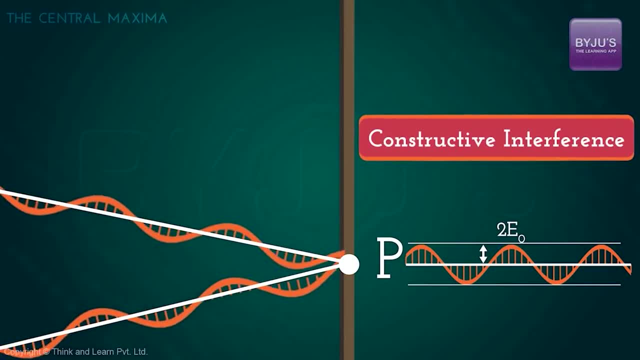 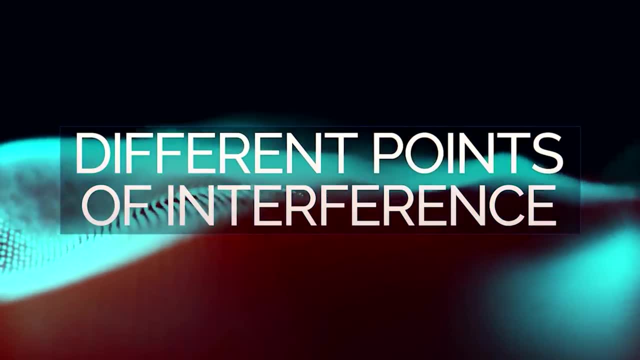 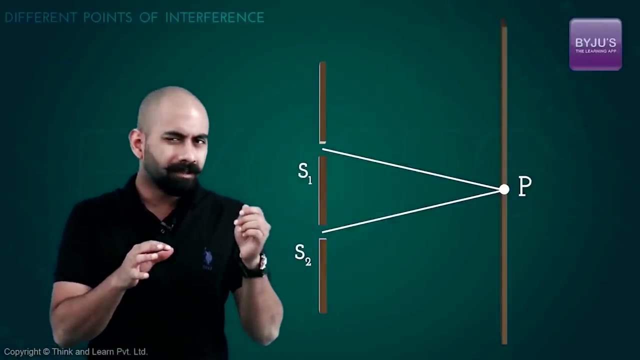 This is obviously constructive interference, right, Because the waves that are interfering, they are in phase, because the path difference is zero. Now let me try something different. What if I move that point P a little up, a little above? Okay, Now what will happen? 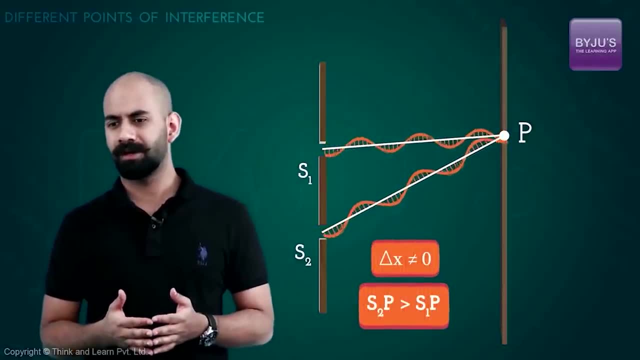 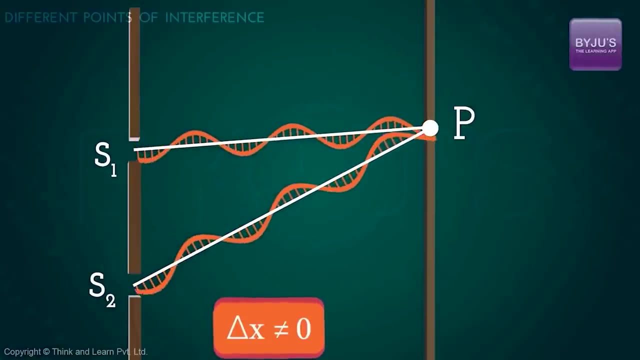 Now, obviously, the path difference will not be zero anymore, right, Because the wave that's coming from S2, the path it's taking will be longer than the wave that's coming from S1, right, So there will be a path difference, which means there will be some phase difference. 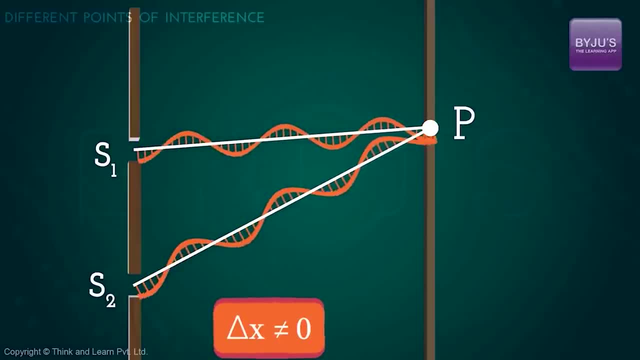 as well. right, And when these two waves interfere, what will be the amplitude? I don't know. That depends on phase difference. Okay, But what if? What if I move it up? What if I move this point P in such way that the path difference equals lambda by 2, right. 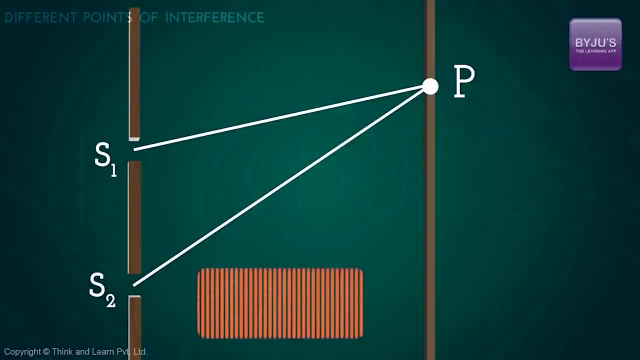 So I move this P up, I bring it to a point such that S2P minus S1P equals lambda by 2. Then think about it. What will happen. So if you can imagine two waves that are coming from S1 and then S2, right, both of them are. 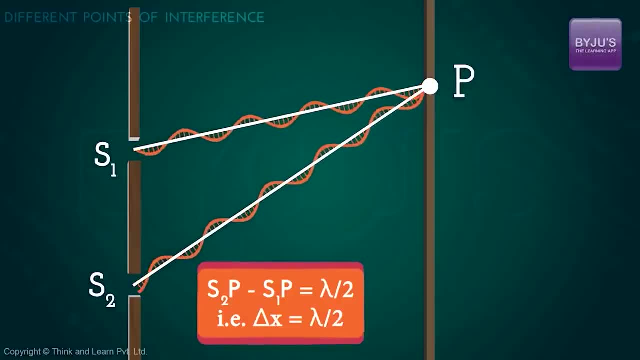 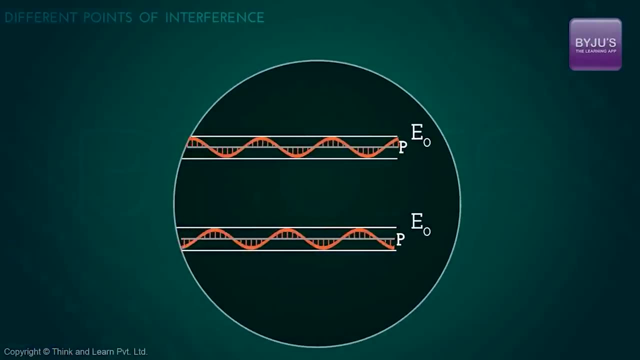 traveling with the same speed. But S2P, basically the wave that's coming from S2, will take a longer time right to reach there, because the time taken, or rather the path, is longer. Okay, So S1P, or the wave that's coming from S1, will reach first, okay, 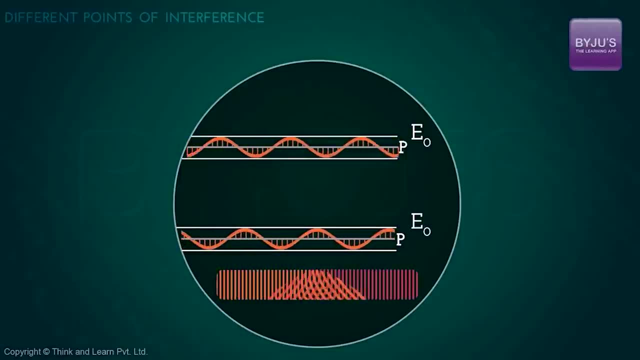 But S2P will reach a little later, but with what difference? With the difference of lambda by 2. That means there will be destructive interference, right? So if you look over there, they'll reach in such a way that the field contributed by the 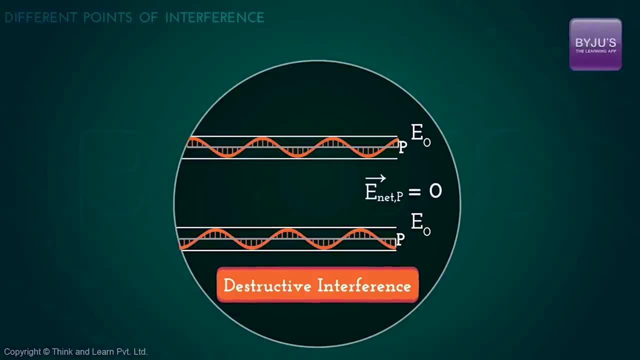 wave from S1 will always be negative of the field contributed by the wave from S2.. Okay, Okay, Okay, So the net field at that point will always be zero, Or the amplitude but at that point will always be zero. So this is destructive interference, okay. 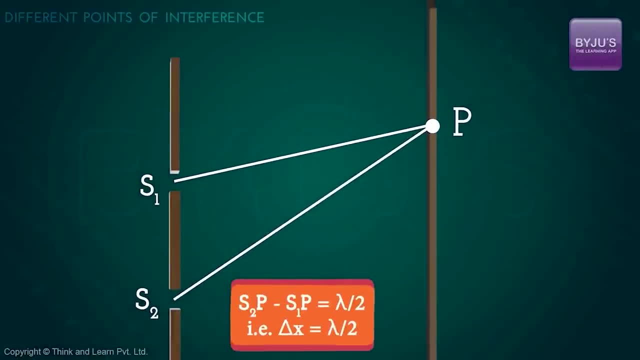 This is interesting. Now wait, what if? okay, let's assume that if I keep moving this point P further and further up, okay, I assume that the path difference will only increase. If I make that assumption, okay, then at a particular point P, again, if I make that, 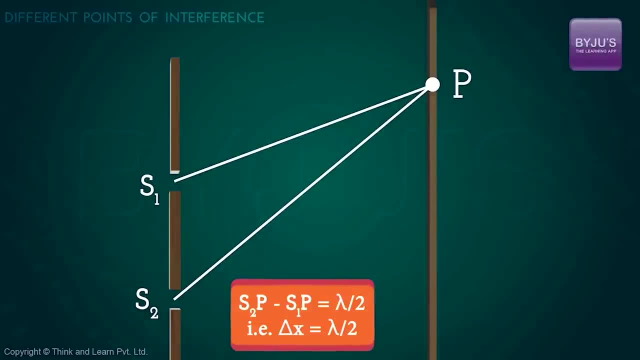 Again, if I move it up, there will be a point where s2p minus s1p equals lambda, right? So that basically means the path difference equals lambda. Then what will happen Then? obviously the wave from s1 will again reach first, but the wave from s2 will reach. 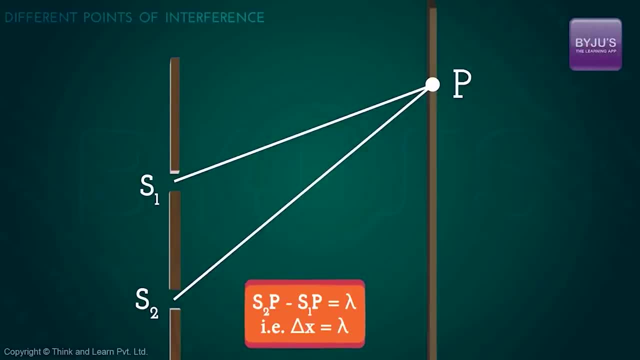 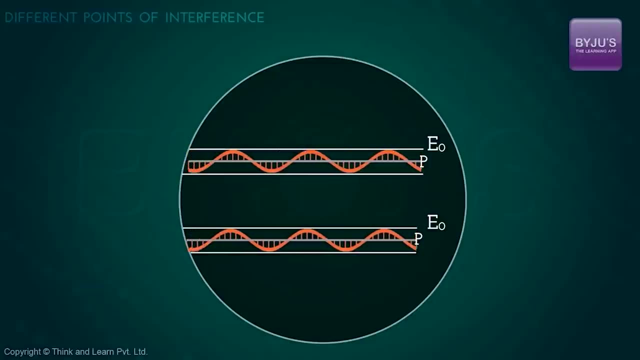 after some time, but just after the first wave has finished, one lambda right, Or basically the phase difference will be 2pi, But we know that this also corresponds to constructive interference. We know that the net amplitude will be 2e0 in this case. 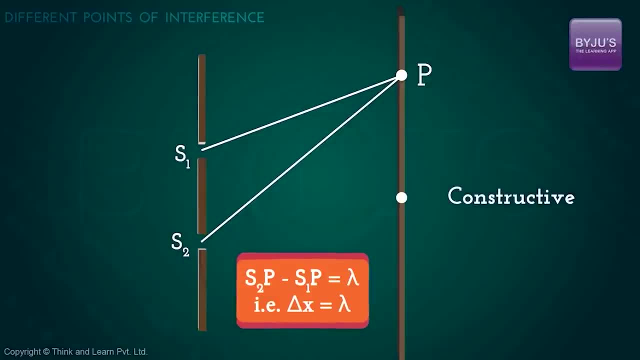 So okay, so that means we will have constructive in the middle, then destructive, then constructive again. Okay, this is interesting. Also, this will be exactly true for the bottom as well. right, If I move instead of moving p up, if I move p down, exactly the same thing will happen. 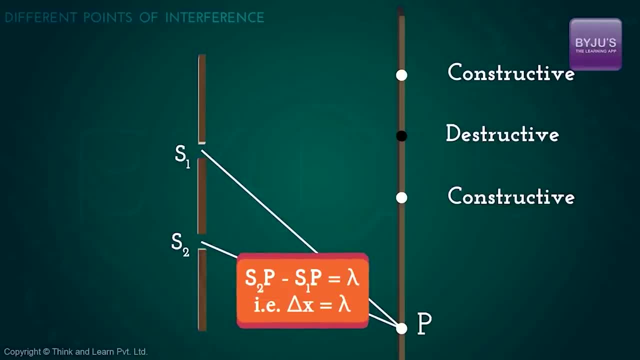 right Because it is symmetric. So there will be a constructive interference, a point with constructive interference exactly at the center. Above that there will be destructive, then constructive. Similarly, below that, there will be one destructive point and then a point with constructive. 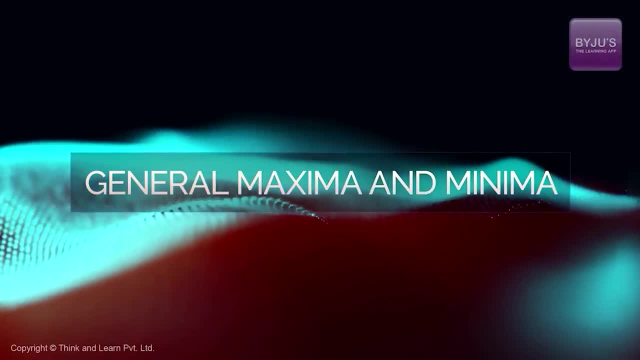 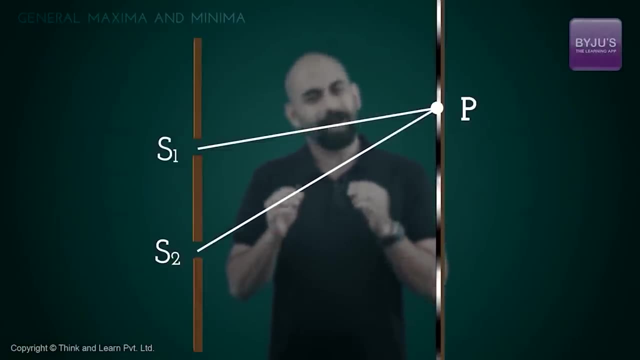 interference. Okay, so now that we know this, let us do something else. Now let us see what happens if I move this point p even further up. Now, if we stick to the assumption that as we move this point p up, the delta x increases, 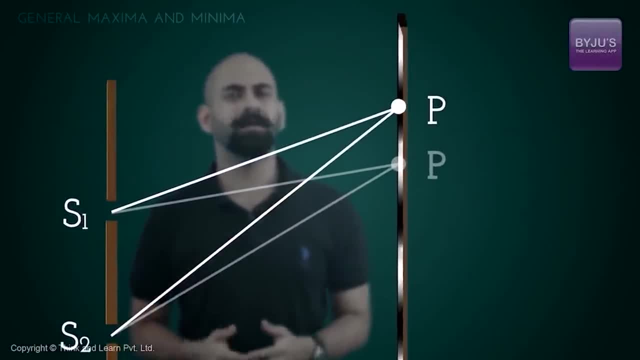 then at some particular point we will have a point p. At some particular point the delta x will become 3 lambda by 2, right? What will happen there Then? that will mean that at that point we will have destructive interference again. 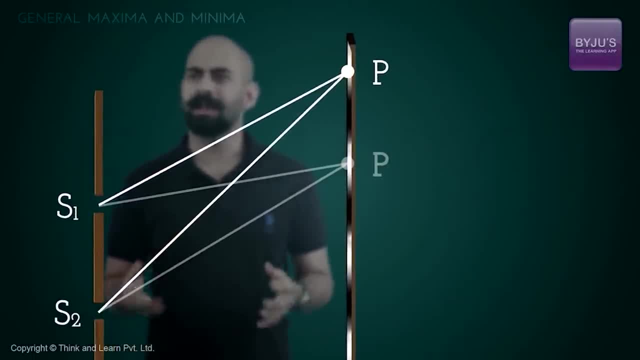 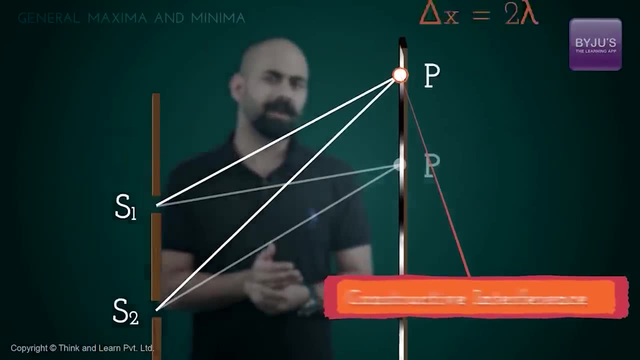 Now, if I do the same thing again, if I move it further up again- delta x- there will be some point where delta x equals 2 lambda. Then at that point we will have constructive interference again, And once again, the same is true below as well, because it is symmetric.